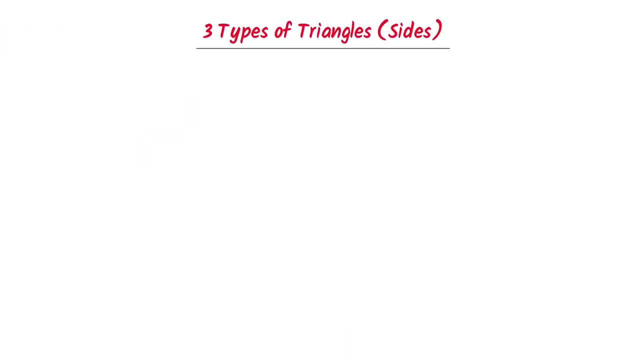 the three types of triangles on the basis of sides. The first type of such triangles are equilateral triangles. In equilateral triangles all three sides are equal. That's why we put single dash on all three sides. For example, in this triangle, this side is 6 cm. this side is. 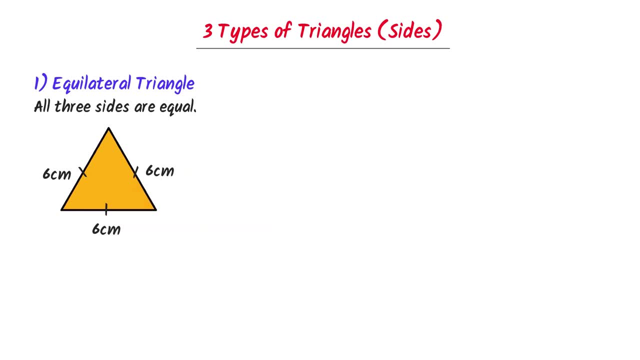 6 cm and this side is also 6 cm. Here all sides are equal, so we call it equilateral triangle. The second type of triangles is isosceles triangle. An isosceles triangle, only two sides are equal. That's why we put single dash on two sides and 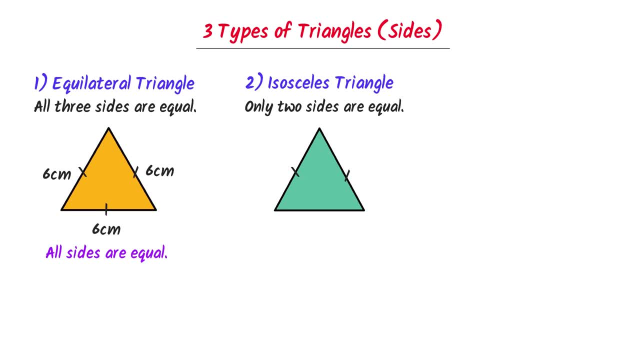 leave the third side. For example, in this triangle, this side is 5 cm, this side is also 5 cm and this side is 7 cm. Here only two sides are equal, so we call it isosceles triangle. 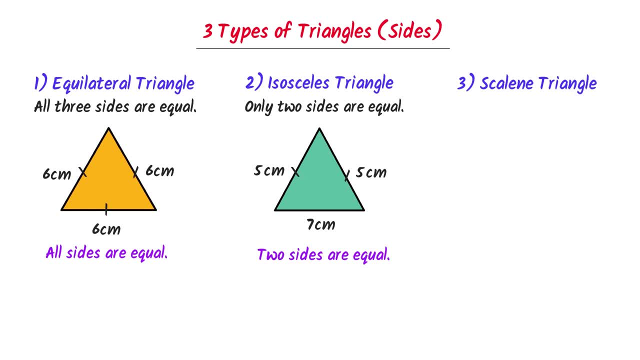 The third type of triangles is scalene triangle. In scalene triangle all three sides are different. For example, in this triangle this side is 5 cm, this side is 7 cm, while this side is 9 cm. Here, all three sides are. 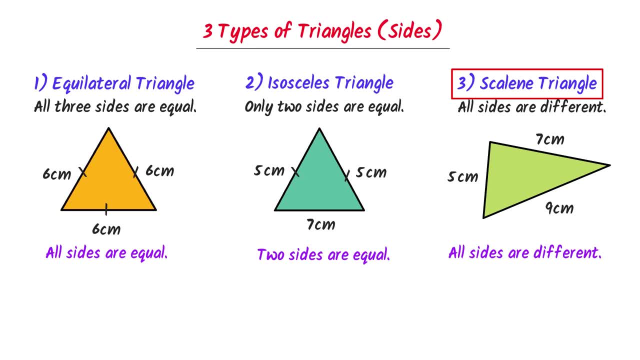 different, so it is scalene triangle. Thus, these are the three types of triangles on the basis of sides. Now here is one important question: How can we remember these triangles, How can we remember the three types of triangles easily? Well, I always teach my personal trick. 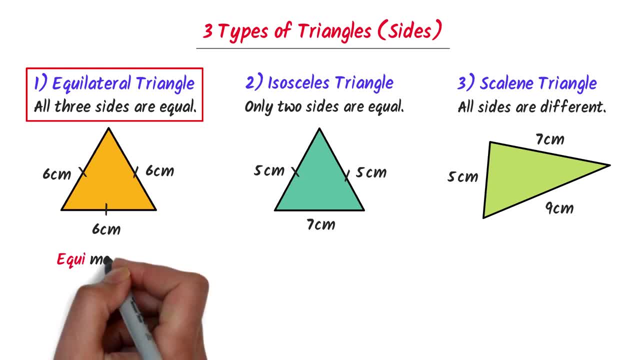 In case of equilateral triangle, the word equi means equal and the lateral means sides, So the word equilateral means equal sides. Therefore, equilateral triangles are those triangles in which all sides are equal. In case of isosceles triangles, and the first, 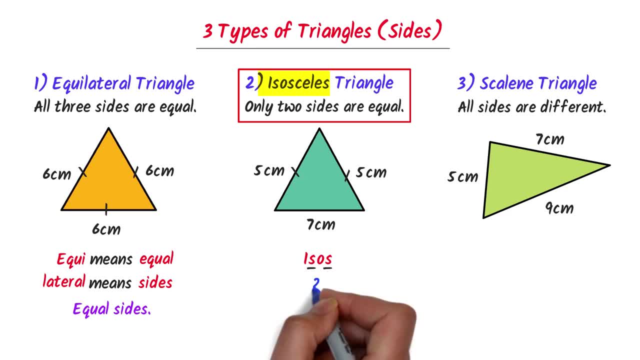 four alphabets there are two s are two times s. So in isosceles triangle two sides are equal. In case of scalene triangle, in the first four alphabets all the four alphabets are different. or we say that there is only one s, which means that not a single side is. 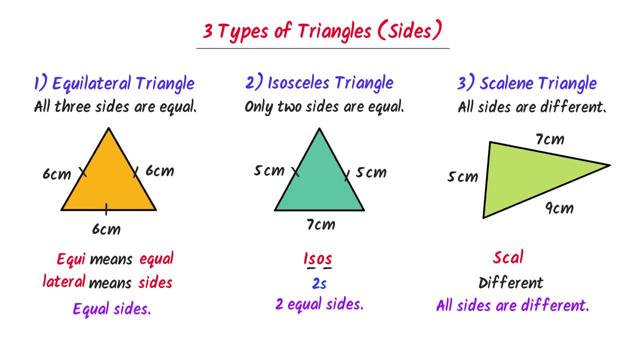 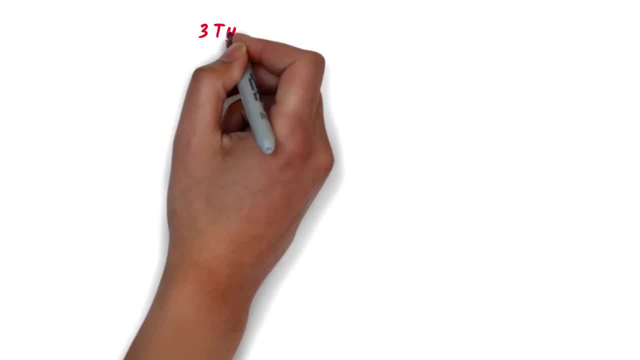 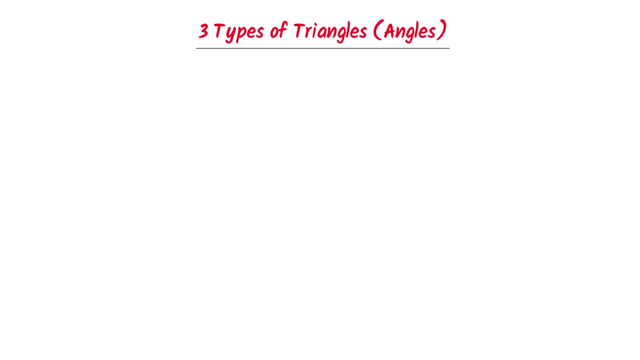 equal or all sides are different. Thus, using this simple trick, we can easily remember the types of triangles. Finally, let me teach you the three types of triangles on the basis of angles. Well, I teach my personal trick. I always write a? r? o? n around. Now below. 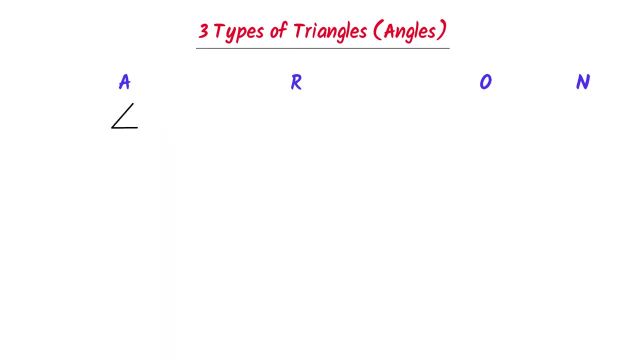 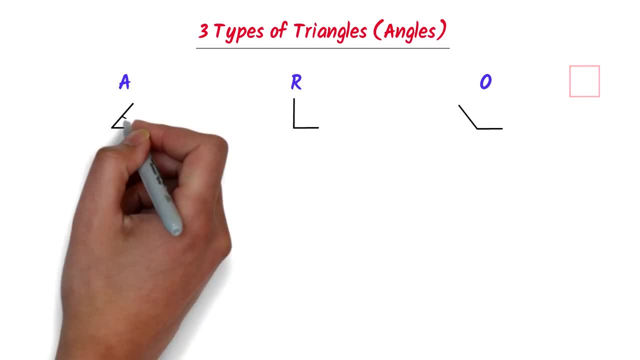 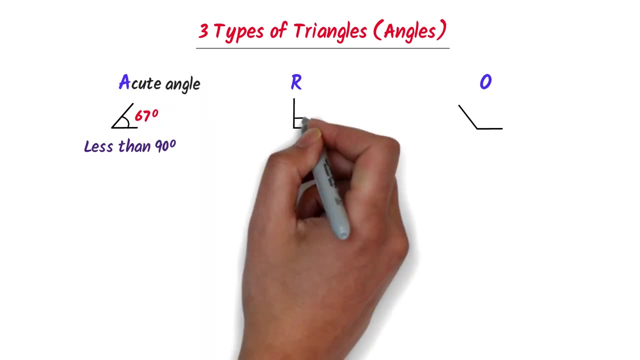 this angle, And I do not draw anything below n. Now, this angle is less than 90 degree, So a stands for acute angle. This angle is equal to 90 degree, So r stands for right angle And this angle is greater than 90 degree, So o stands for obtuse angle. Now on the 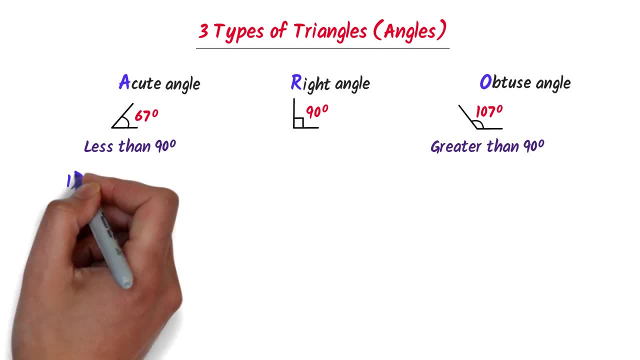 basis of angles. the first type of triangle is acute triangle, Those triangles in which all the angles are like this, So r stands for acute angle. Now, on the basis of angles less than 90 degree are called acute triangles. For example, in this triangle, this angle 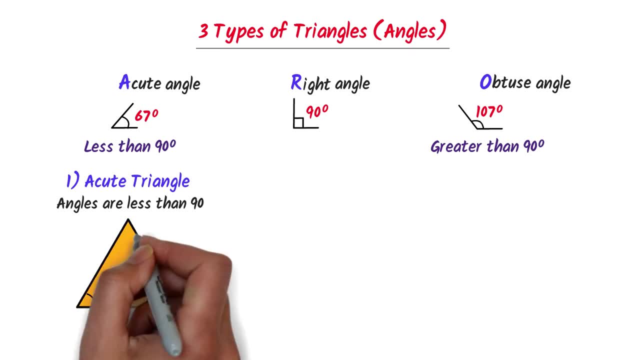 is 50 degree. This angle is 70 degree. This angle is 60 degree. Here all the angles are less than 90 degree, So it is acute triangle. The second type of triangle is right triangle, a right angled triangle, Those triangles in which one angle is 90 degree, a right angle. 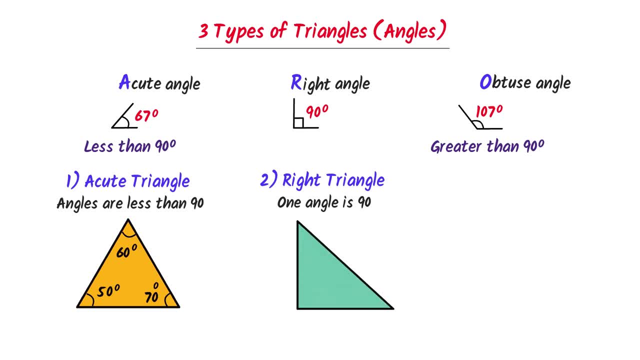 are called right triangles. For example, in this triangle this angle is 90 degree, So this triangle is known as right angle, a right angled triangle. The third and the last type of triangles is obtuse triangle. Those triangles in which one angle is obtuse angle are called 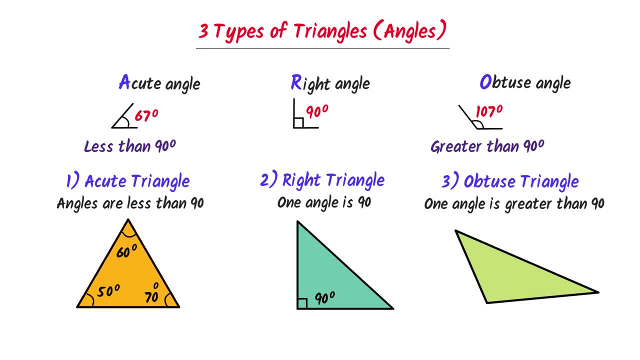 obtuse triangles. For example, in this triangle, this angle is 100 degree, This angle is 90 degree, This angle is greater than 90 degree. So we say that this triangle is obtuse triangle. Thus, these are the six different types of triangles.